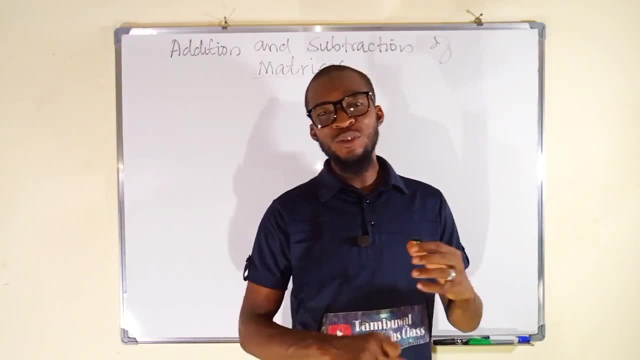 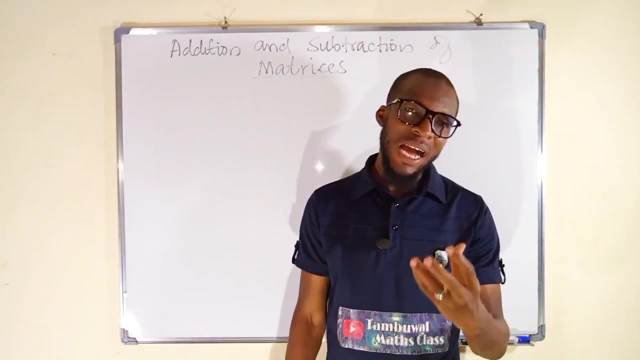 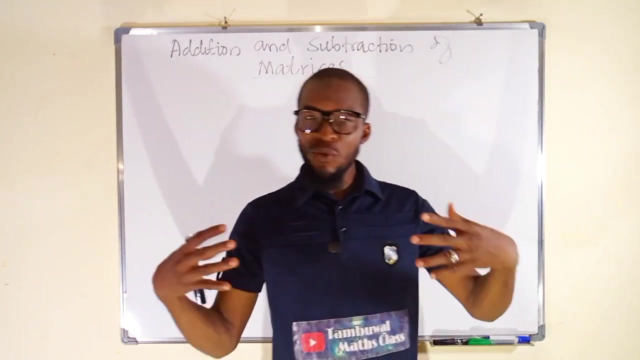 Hello, good day viewers. in this tutorial we are going to look on to addition and subtraction of matrices. But mark you, you can only add or subtract matrices of the same dimension. and what do we mean by this dimension is the number of rows and columns in that matrix. 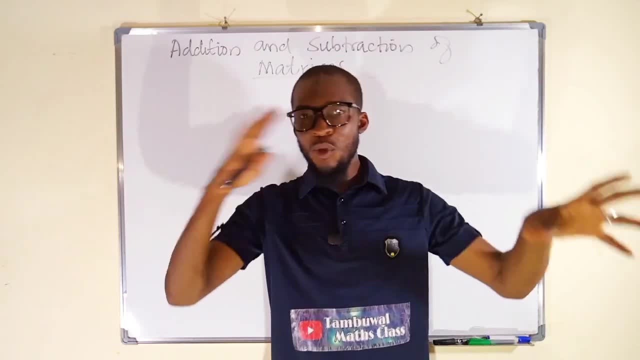 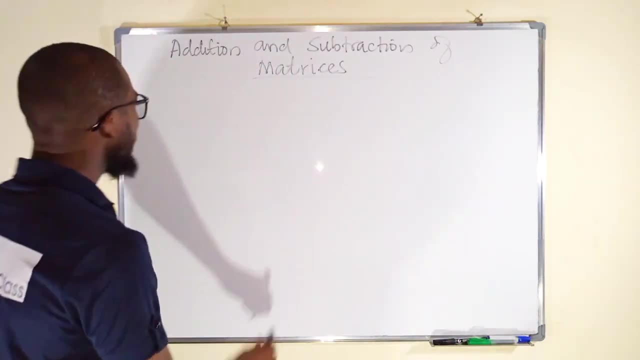 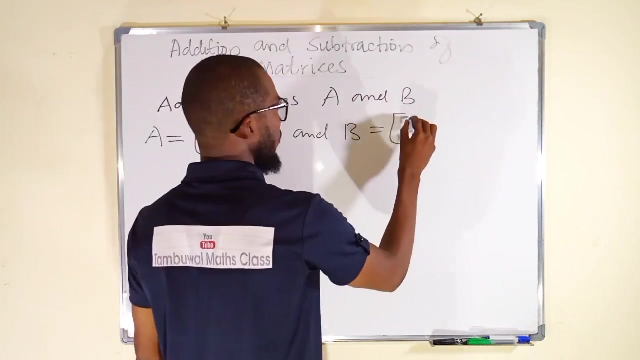 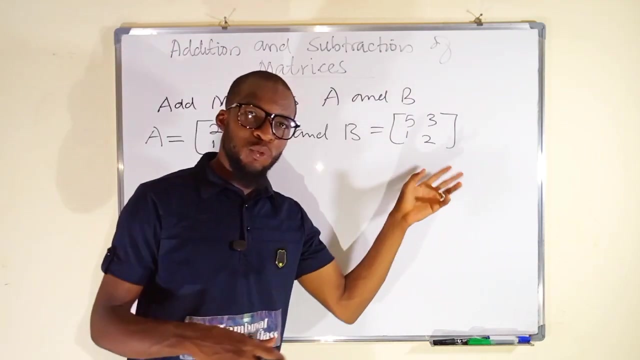 So the number of rows and columns of two or more matrices must be the same for you to add or subtract them. Okay, let's get started. Example: let us add a matrix A and B. You can see these two matrices are of the same dimension, two by two matrices. So how? 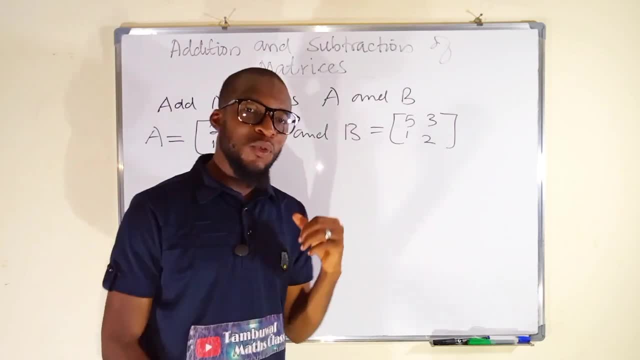 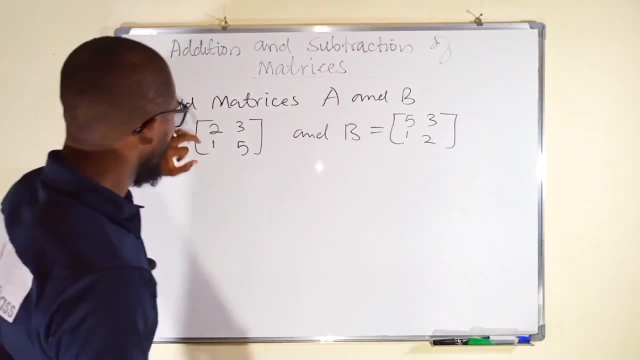 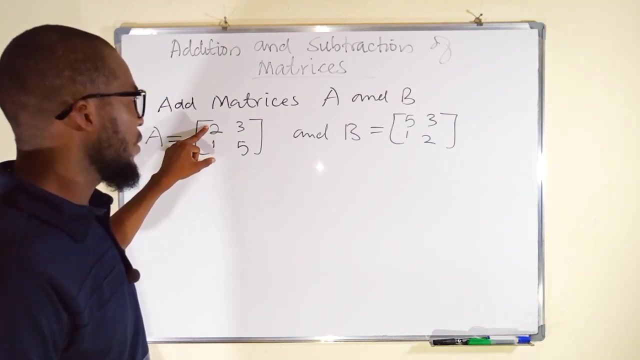 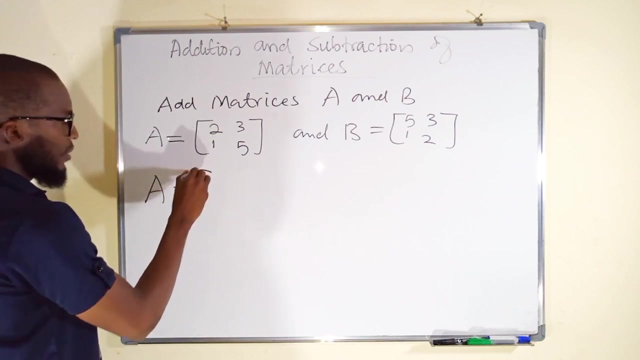 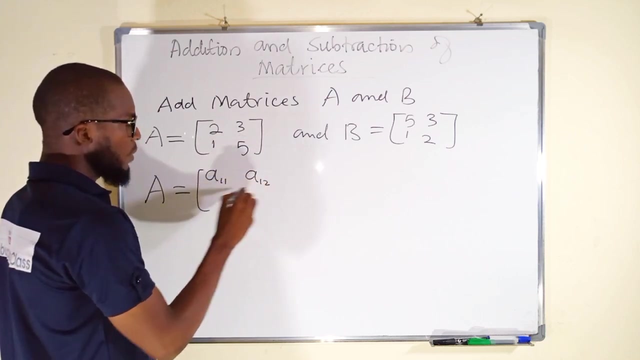 can we add them? To add them, you must add an element to its corresponding element to the other matrix Two. here, the position of these two is at A11.. This is B11.. Okay, let me represent them. This is A, The four matrices. let us represent them. We have A11.. This is A12.. A21. A22.. While this is A23.. This is A24.. This is A25.. This is A26.. This is A27.. This is A28.. This is A29.. This is A30.. This is A31.. This is B21.. This is B22.. 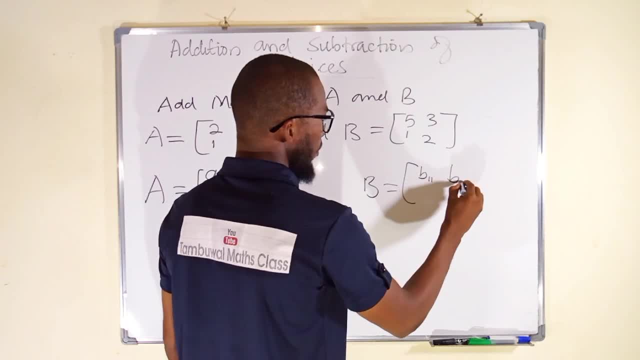 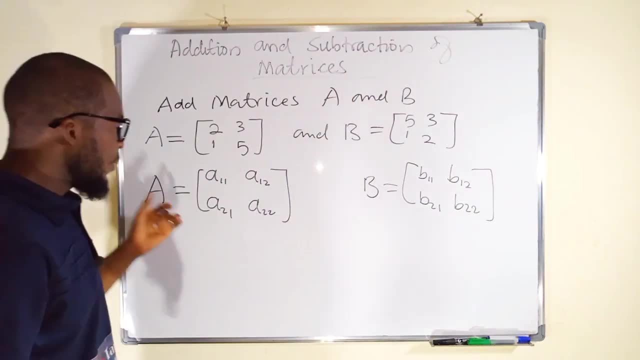 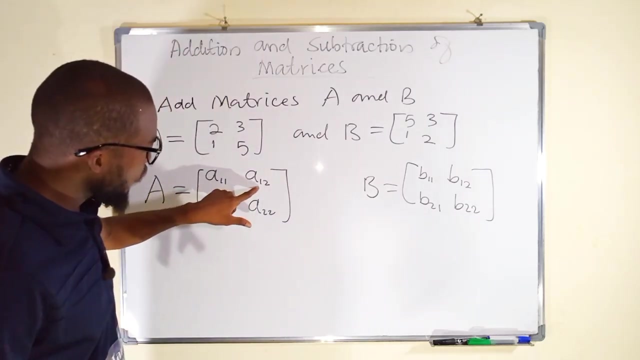 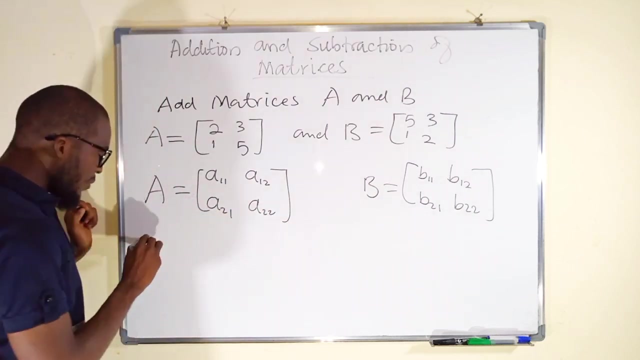 And then the matrix: B11.. This is B21.. This is B22.. This is B21.. This is B22.. You know, these subscript numbers are here to represent number of rows and columns. This is row 1, column 1, row 1, column 2, row 2, column 1, row 2, column 2.. So to add: 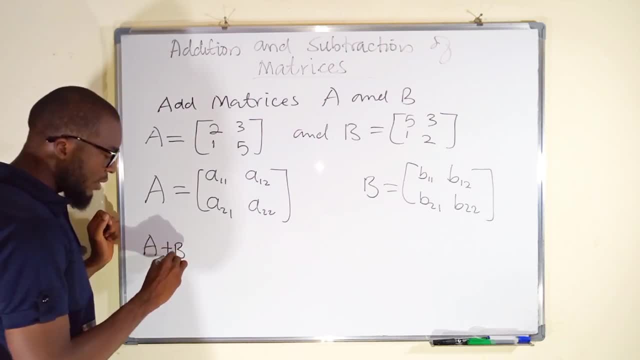 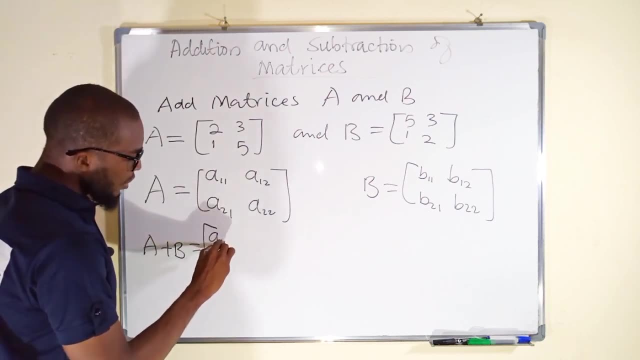 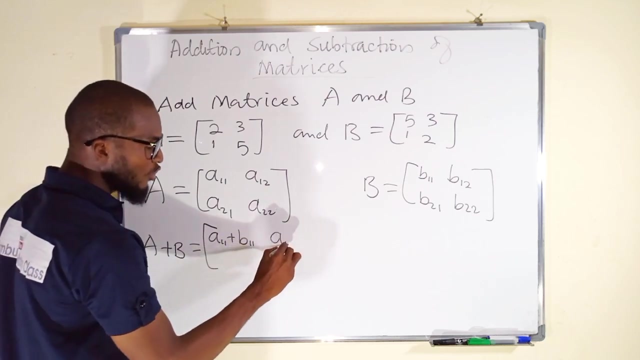 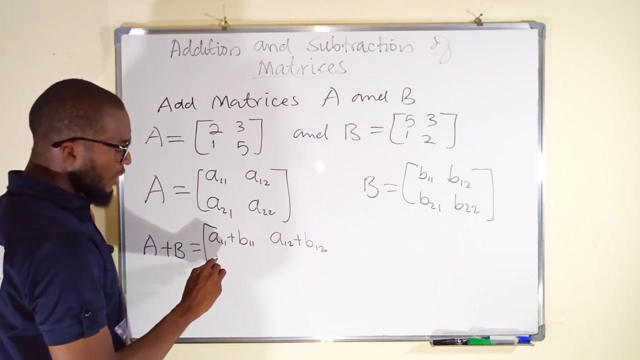 A and B- A plus B- C and B, C and B. you must add their corresponding elements. so we add a 1- 1 and b 1- 1 together. then you give a space, you add a 1- 2 and b 1- 2 together. then you come here. you add a 2- 1 and b 2- 1 together. 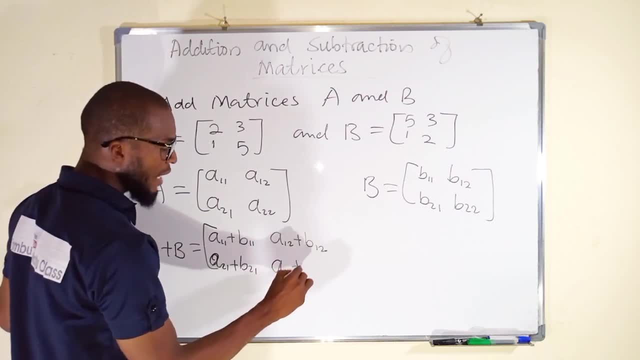 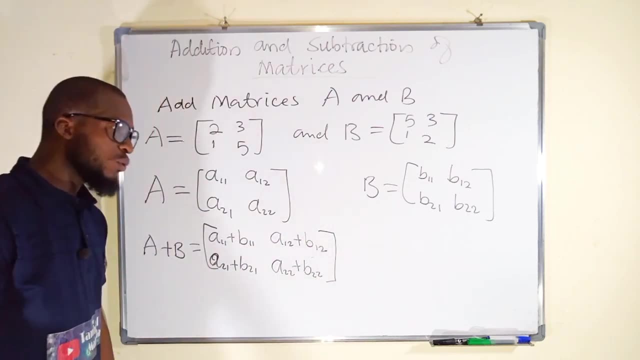 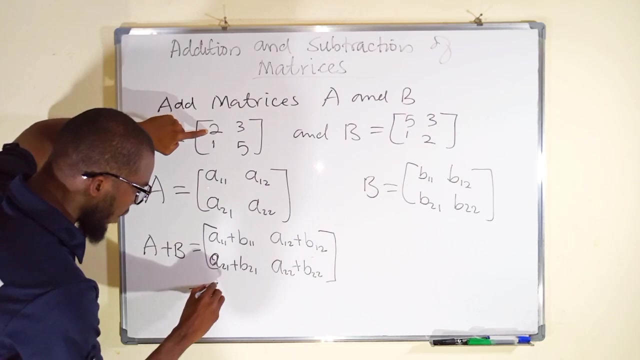 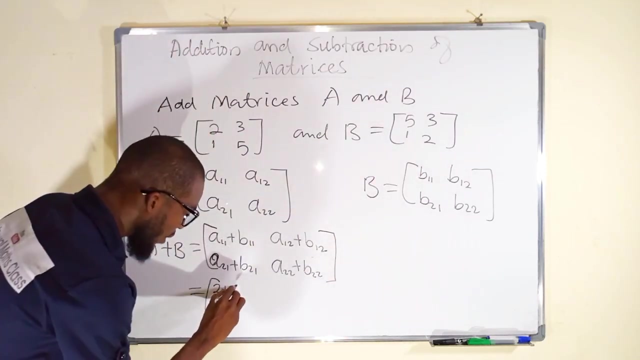 add a 2- 2 and b 2- 2 together. this is how you'll do it. okay, now let us substitute a 1, 1 is 2 here. you can see it. so we have 2 plus b 1. 1 is equal to 5, so we have 5 here. then we move: a 1, 2 is 3. 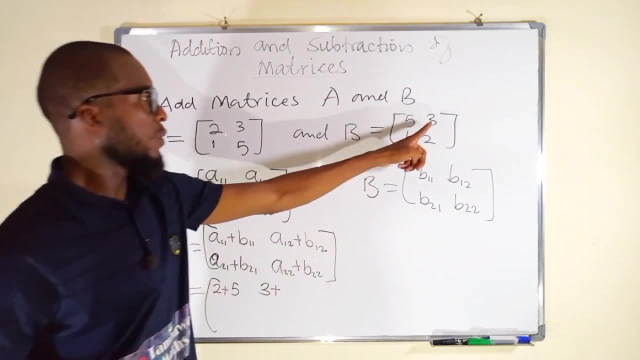 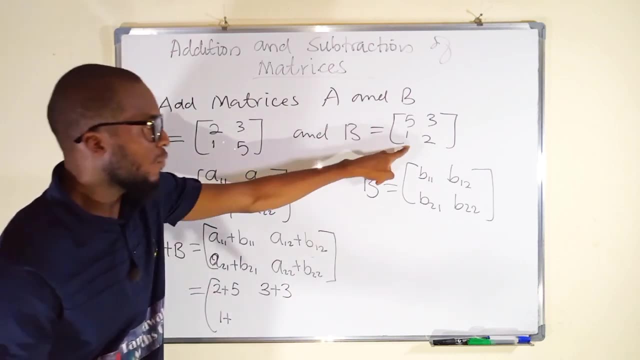 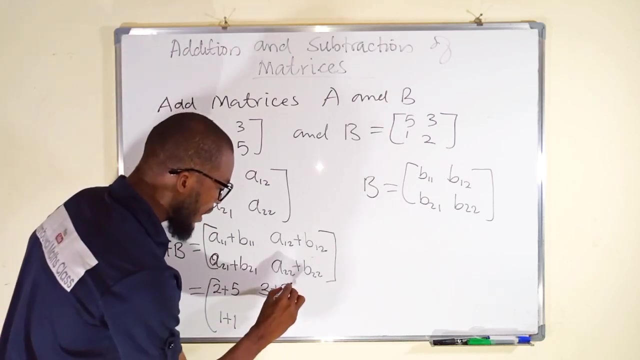 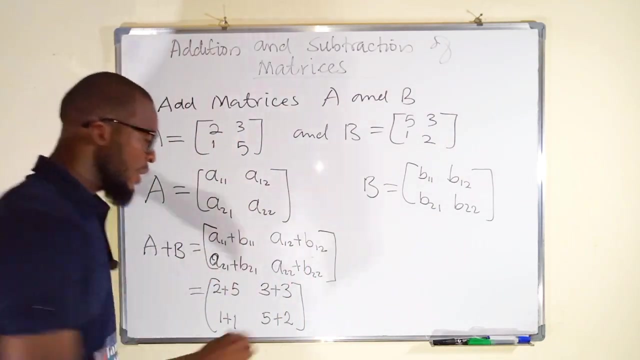 so we have 3 plus we equally have 3 there. we have 1 plus we have 1. also we have 5 and we have 2 to the other side. you must add them together with their corresponding element at the same position. so this is equal to, if you: 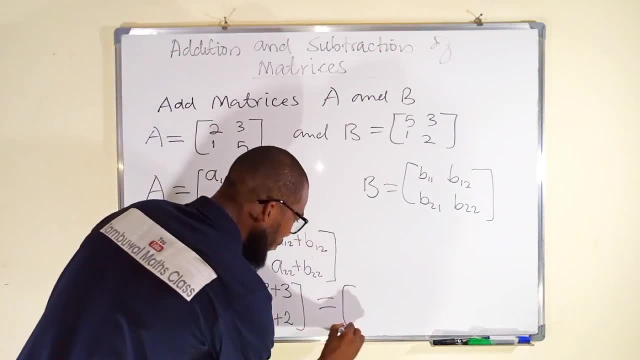 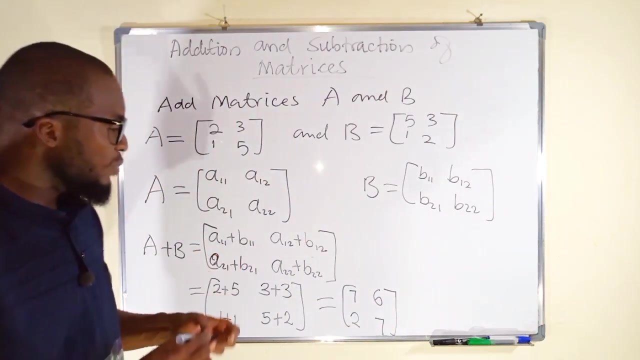 simplify: we have 2 plus 5 equal to 7, and 3 plus 3 is equal to 6, 1 plus 1 equal to 2, pi plus 2 is equal to 7. so by adding matrix A and matrix B, we are able to. 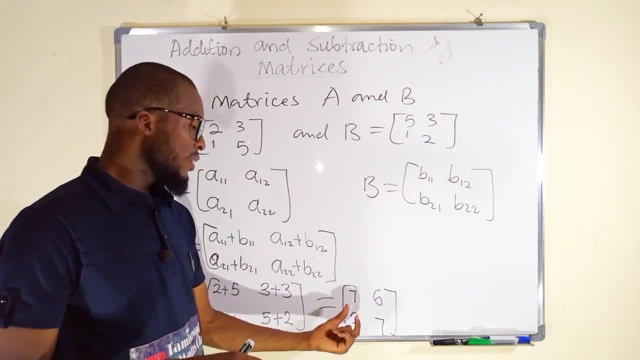 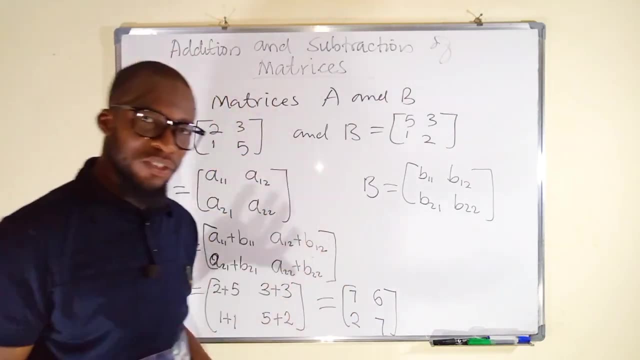 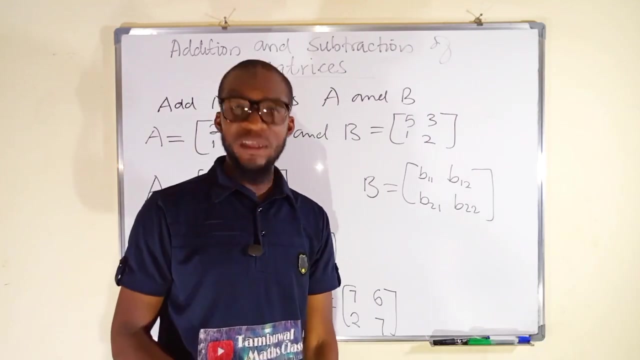 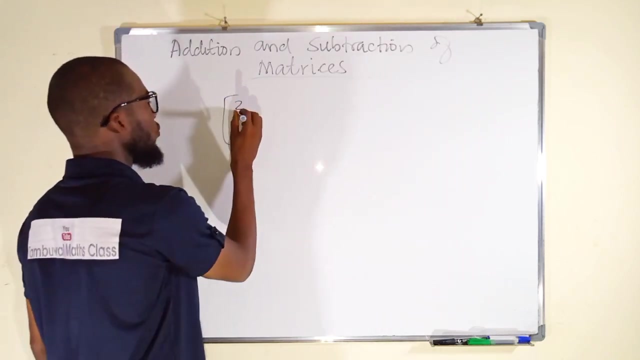 obtain another single matrix: 7, 6 to 7. so this is how to add matrices: you must make sure that they are of the same dimension. number one, number two: every element is to be added to its corresponding elements. let us take another one. so first we want to add 3 by 3 matrices: 2, 1. 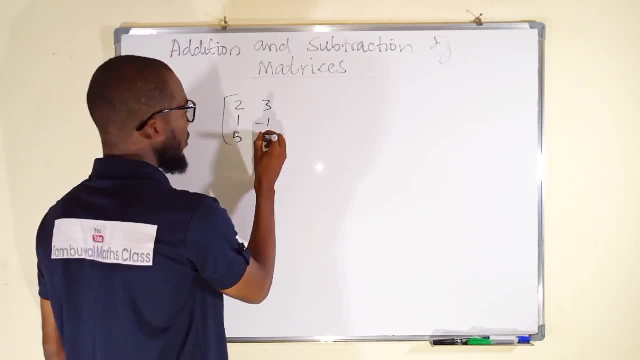 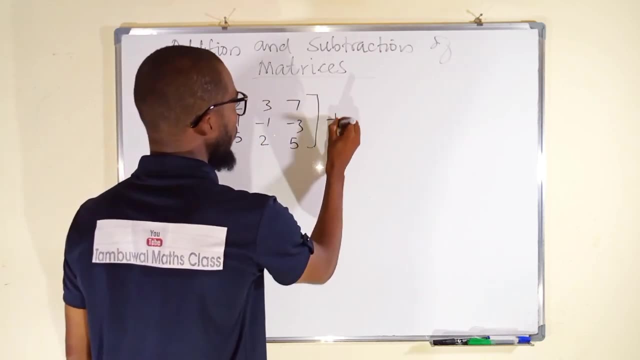 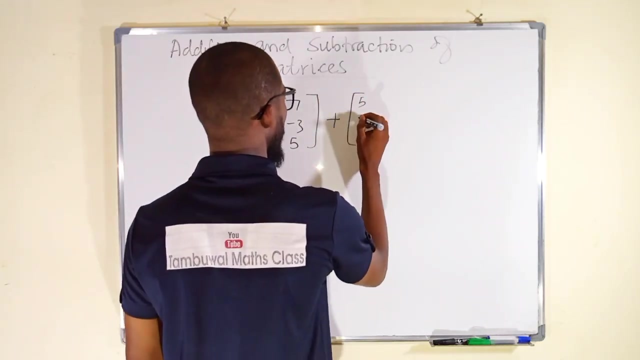 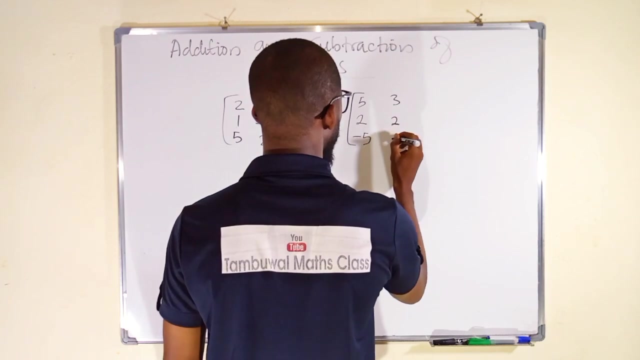 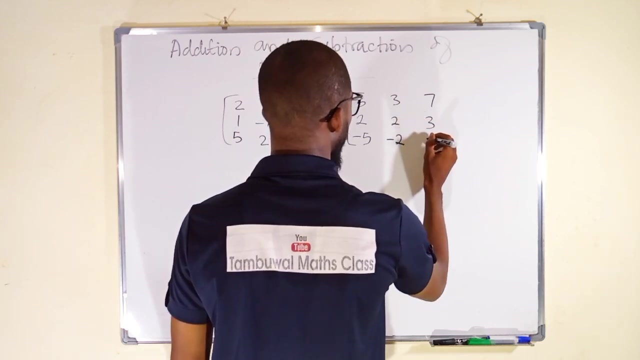 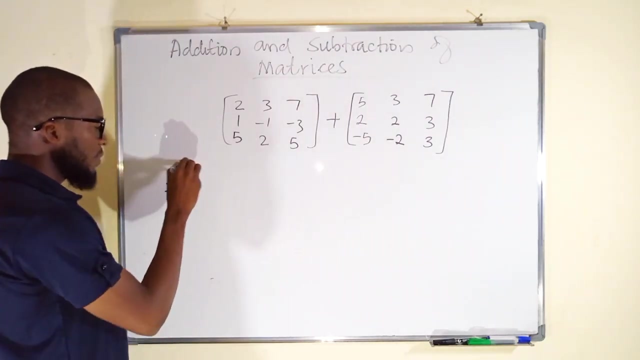 5, 3 negative, 1, 2, 7 negative, 3, 5, together with another matrix also 3 by 3, 5, 5, 2 negative, 5 of 3, 2 negative, 2, 1 of 7, 3 and 3, so now let us add them together. 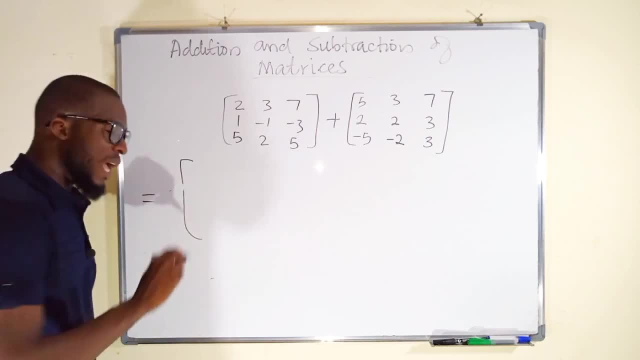 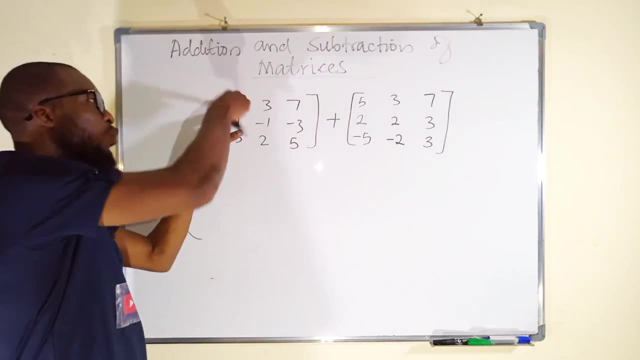 remember what I told you: every element must be added to each corresponding element. we have two here and three here, so now let us add them together. remember what I told you: every element must be added to each element. we have two here at federal column, one festival column. one is 5, so we 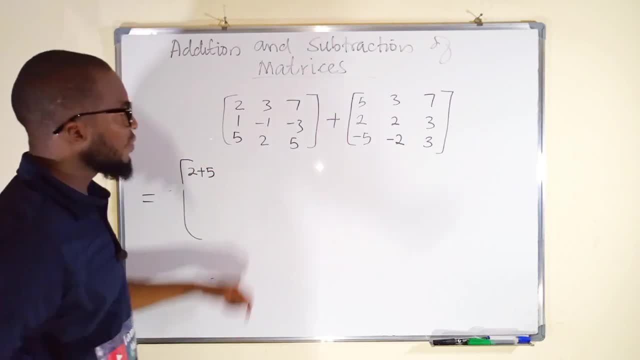 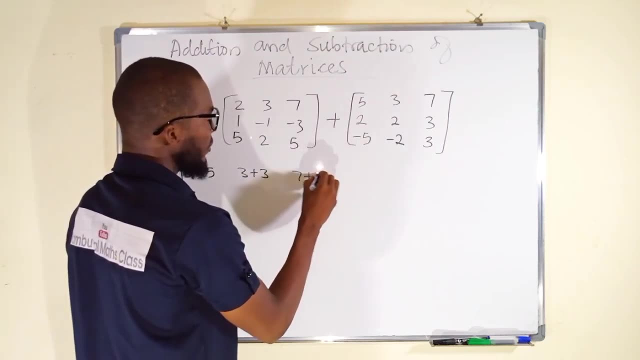 have 2 plus 5. there, you give us this, we have 3 plus 3, 3 plus 3, you move, we have 7 plus 7. second row, we have 1 plus 2. we have negative 1 plus 2. negative 1 plus 2. 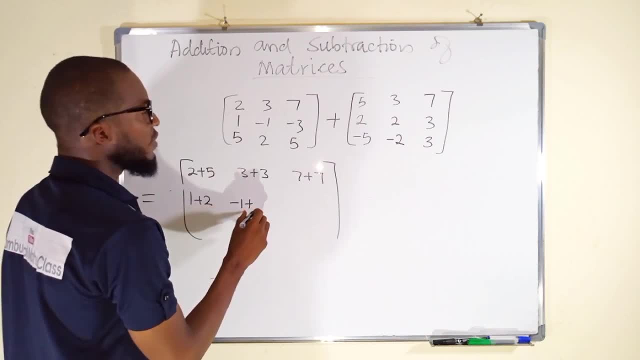 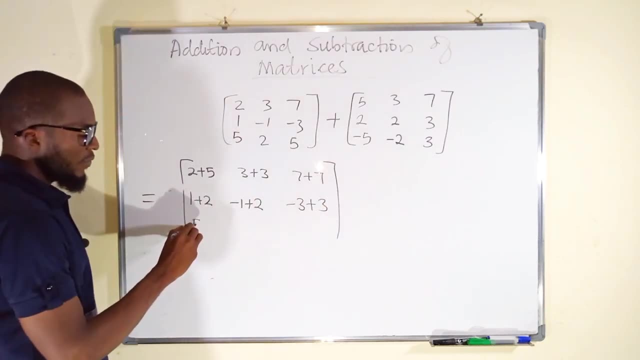 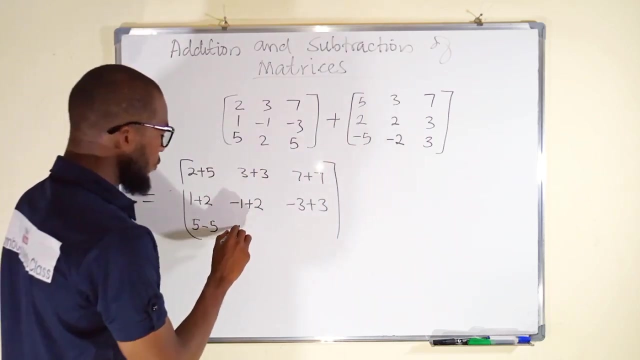 no, okay. so 1, 1, 5 будете 1, niew good plus 1 plus 2, 2. We have negative 3 plus 3.. We have 5 plus, but minus is stronger. We use minus instead. 2, also minus 2.. 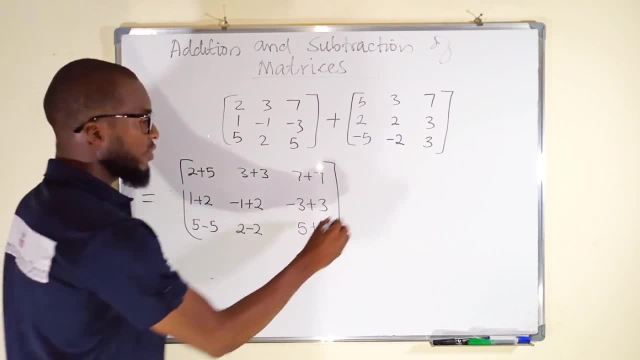 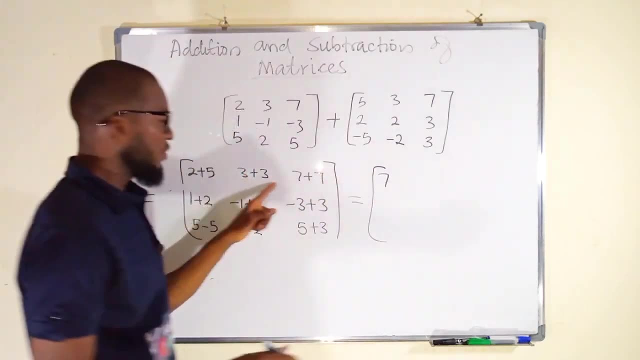 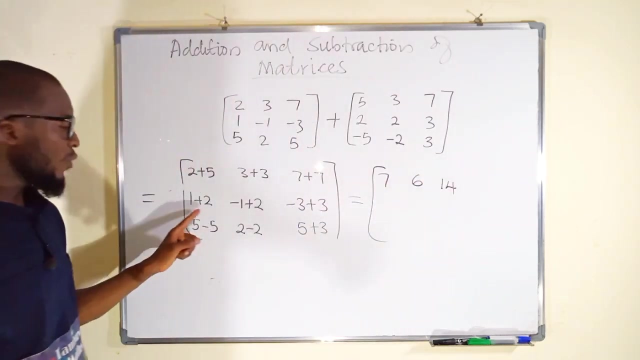 Then 5 plus 3.. Let us simplify and obtain our final result: 2 plus 5 is 7.. 3 plus 3 is 6.. 7 plus 7 is 14.. Second row we have: 1 plus 2 is 3.. 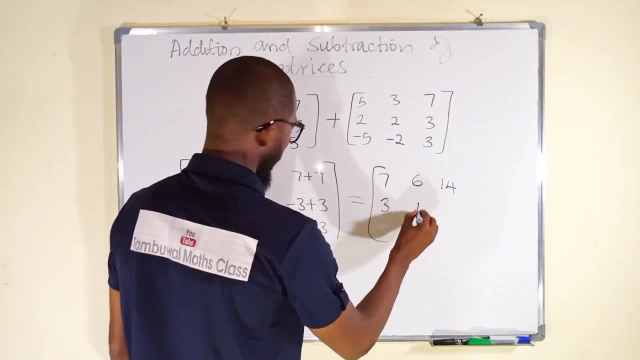 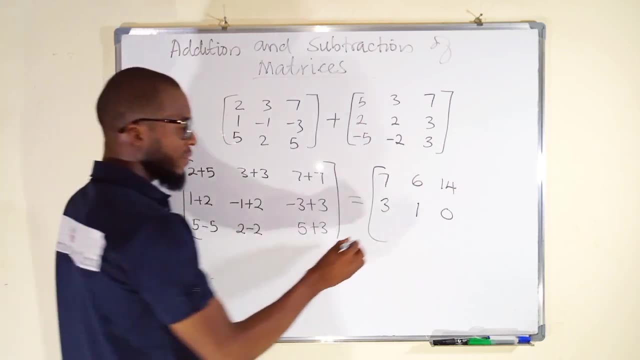 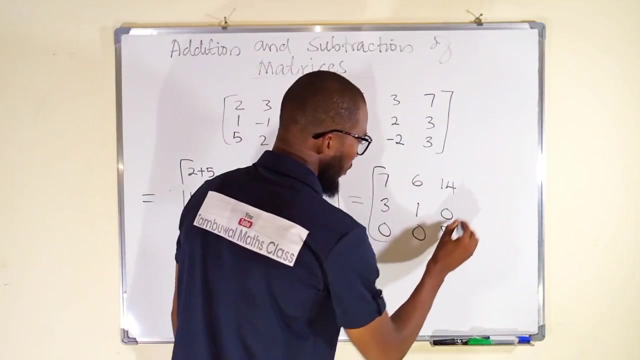 We have negative: 1 plus 2 is 1.. Negative: 3 plus 3 is 0.. 5 minus 5 is 0.. 2 minus 2 is 0.. 5 plus 3 is 8.. So this is the result after adding this to matrix. 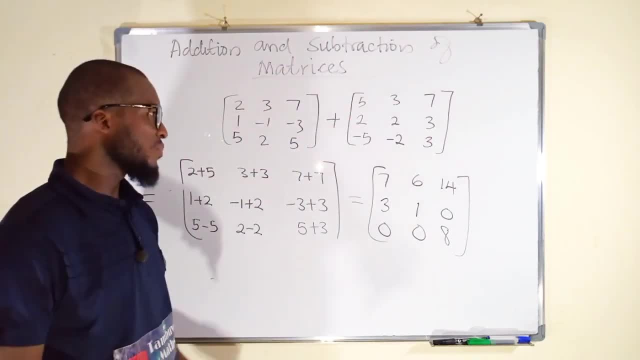 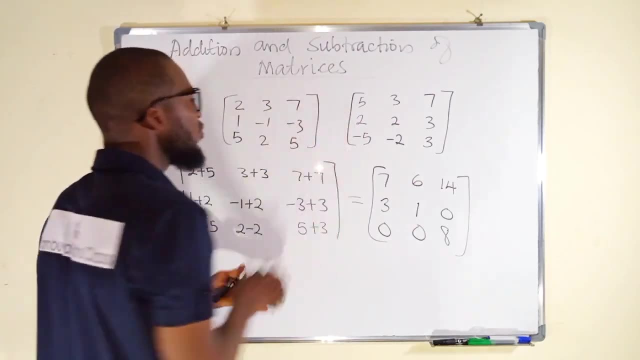 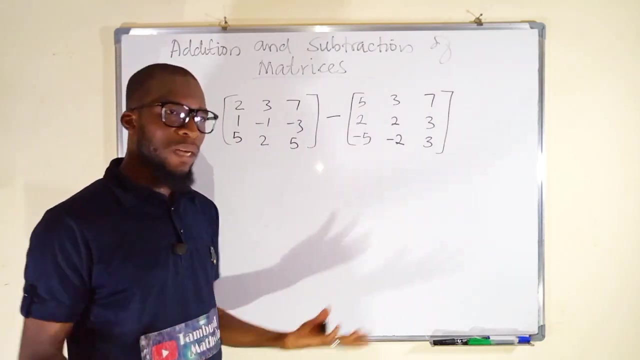 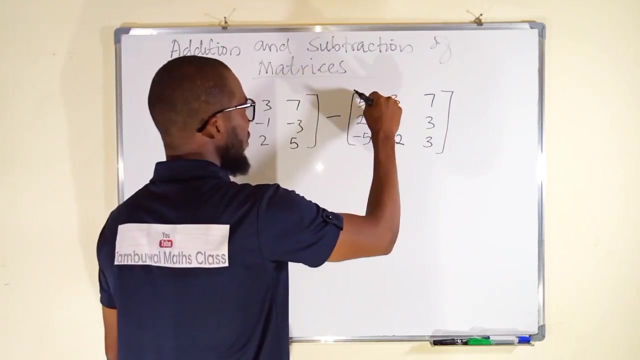 Let us look on to subtraction. Let me just use these two matrices. Suppose we want to subtract instead of adding. To subtract this matrix from this. we follow the same pattern. This element here is at row 1, column 1. You have to subtract this from that. 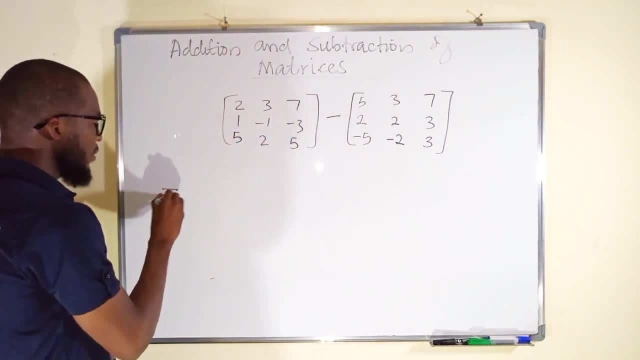 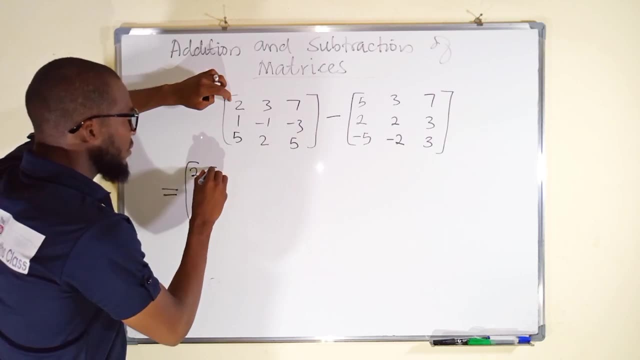 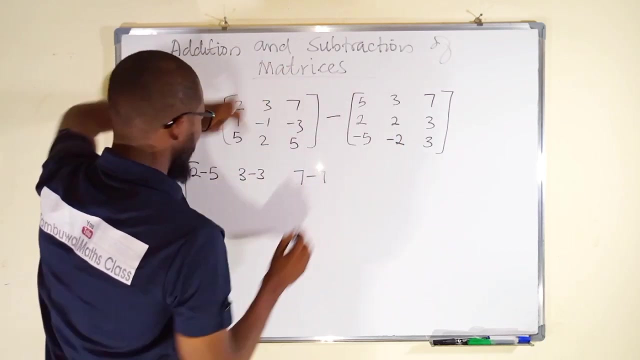 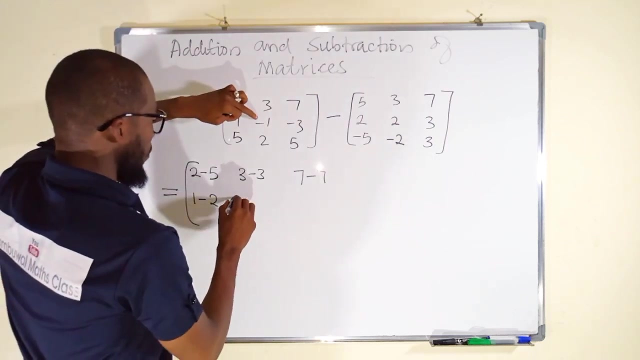 This is what we are going to obtain: We have 2 minus. instead of addition, We have 3 minus 3.. 7 minus 7.. Second row: we have 1 minus 2.. Then minus 1 minus 2.. 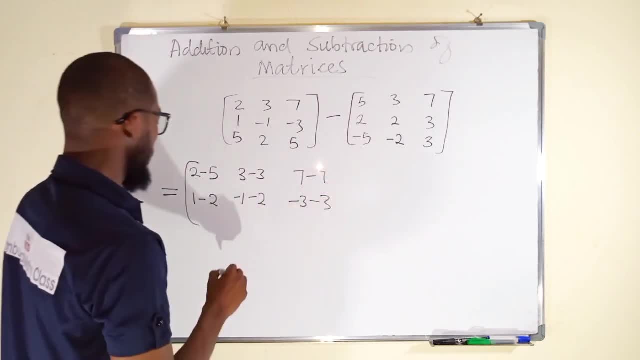 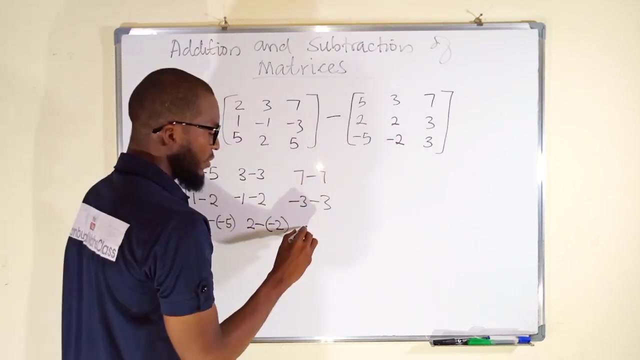 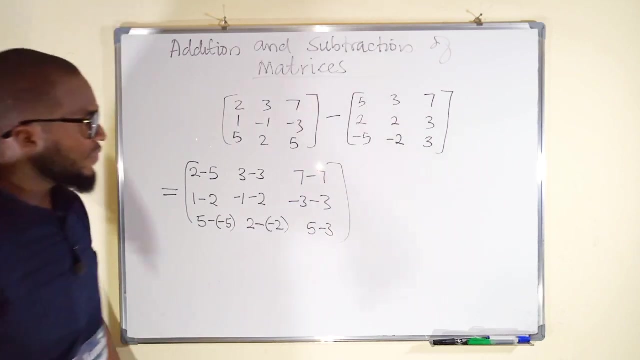 Minus 3 minus 3.. Then the last row is 5 minus minus 5.. We have 2 minus minus 2 and 5 minus 3.. Let us simplify and obtain our final result: 2 minus 5 is negative 3.. 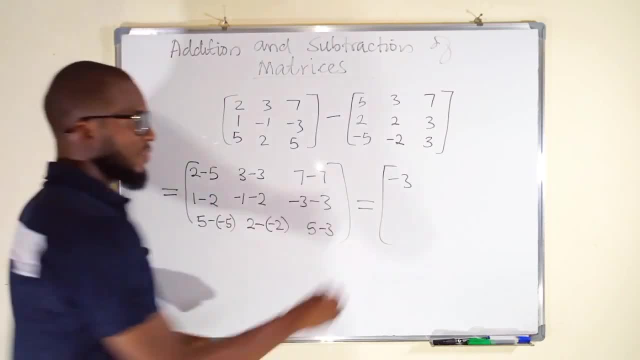 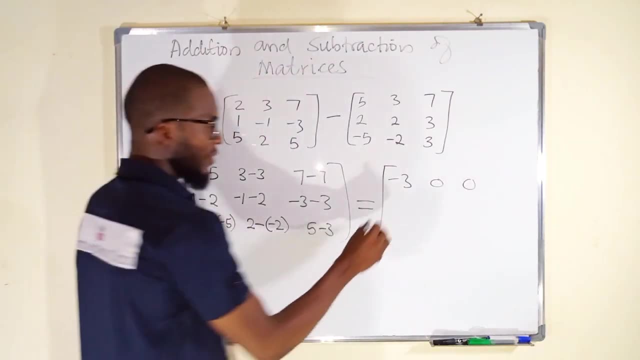 So we have negative 3 here. 3 minus 3 is 0.. So we have 0 here. 7 minus 7 is also 0.. 1 minus 2 is negative 1.. Minus 1 minus 2 is minus 3.. 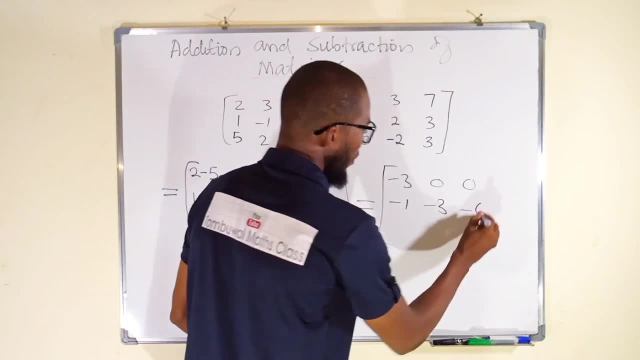 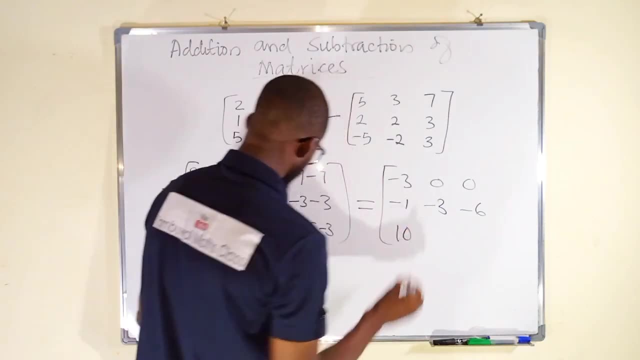 Minus 3 minus 3 is minus 6.. Minus minus is plus 4.. 5 plus 5 is 10.. Minus minus plus 2 plus 2 is 4.. 5 minus 5 is 10.. 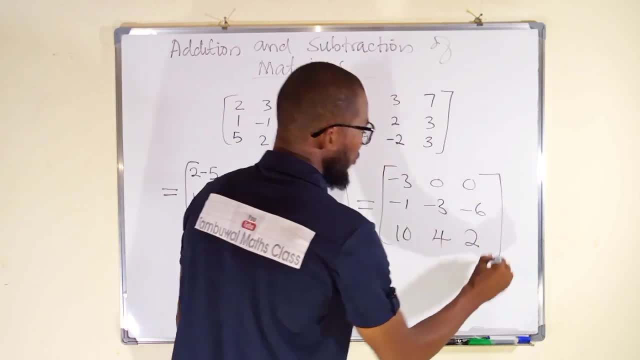 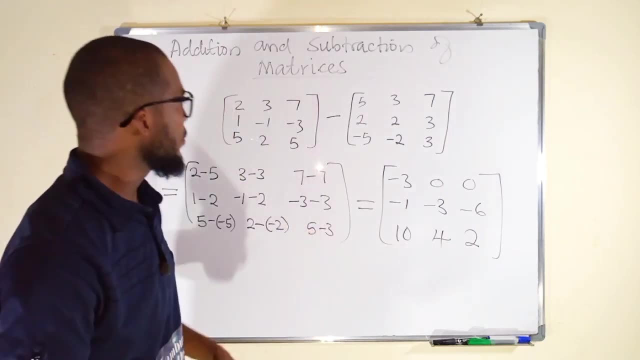 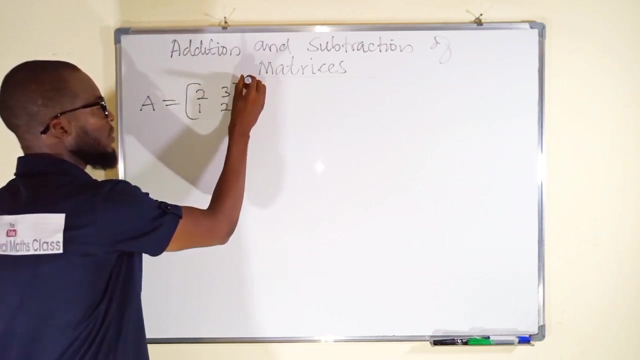 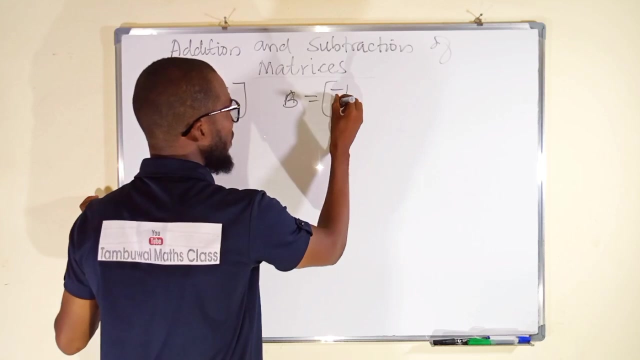 5 minus 3 is 2.. So this is the result after subtracting this matrix from this matrix. Let us take one more example. Let a matrix, A, be 2, 1,, 3, 2.. Let B be another matrix of minus 1,, 3,, 2 and 5.. 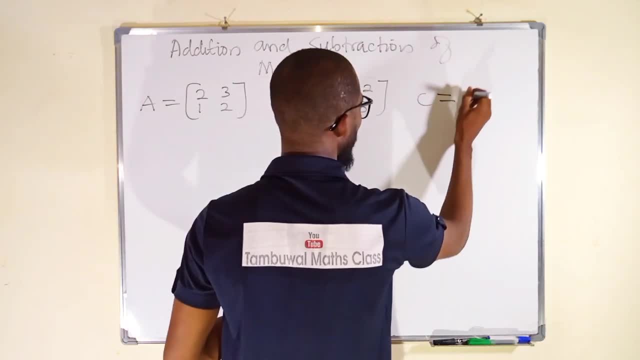 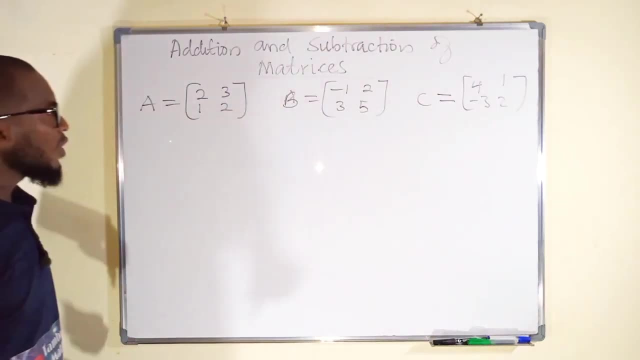 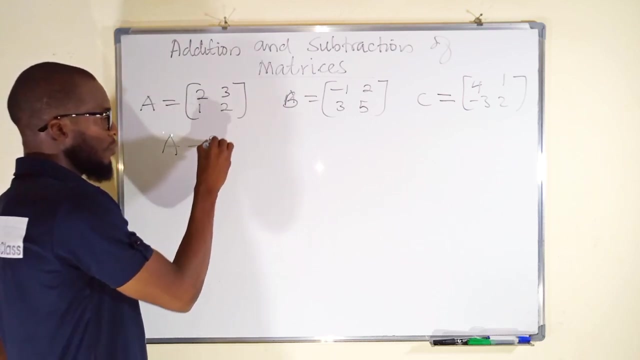 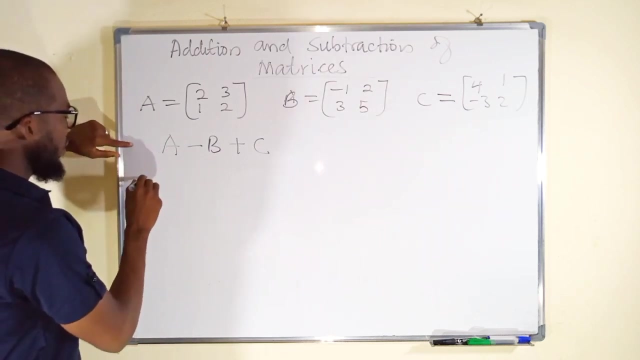 Another matrix, C, to be equal to 4, minus 3, 1 and 2.. Let us form a question here. We want to say A minus B plus C. We want to form a matrix of this form. This is going to be for A. we have. 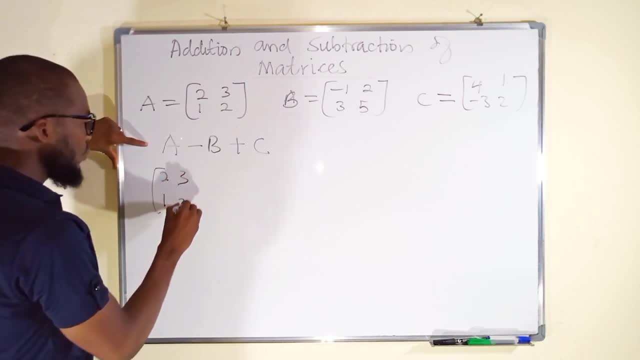 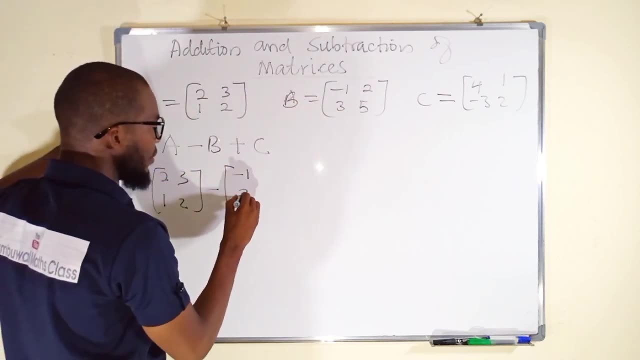 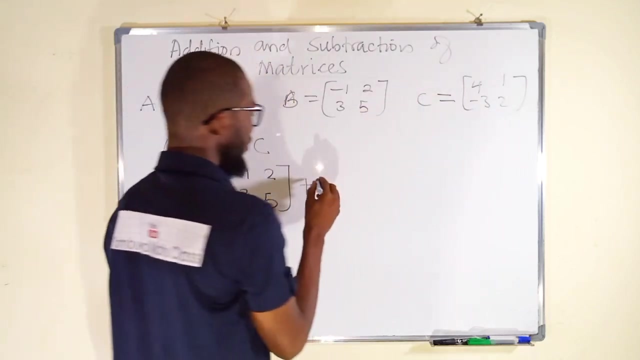 2,, 1,, 3, 2.. Minus sign: we have B Minus 1,, 3,, 2, 5.. Then the last one. we add this matrix: 4, negative 3, 1 and 2.. 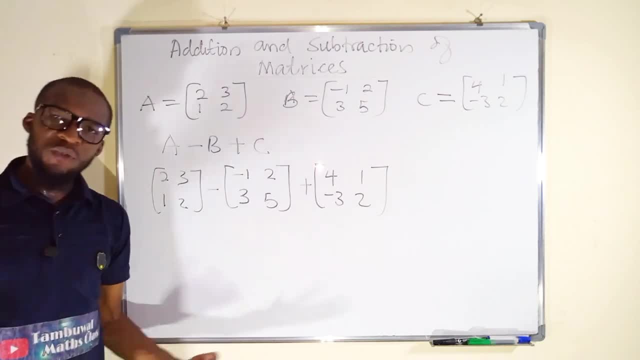 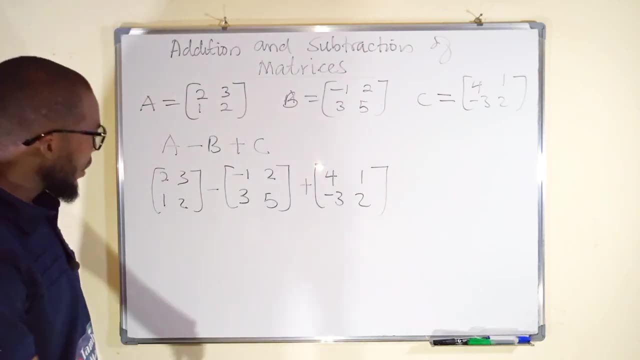 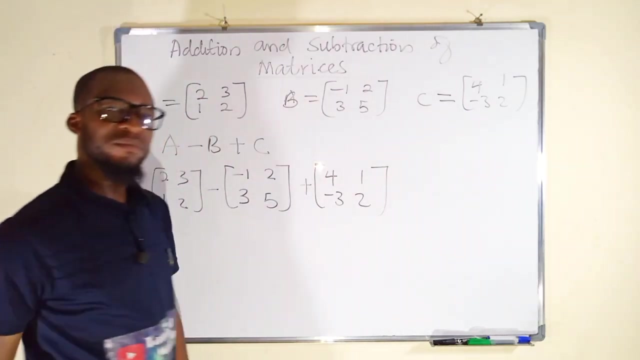 Now we can do it anyhow, If we like. we can add these two matrix, Then we subtract from the first matrix. We can as well subtract this from this, The result we add to this, Or we can carry them simultaneously All together. 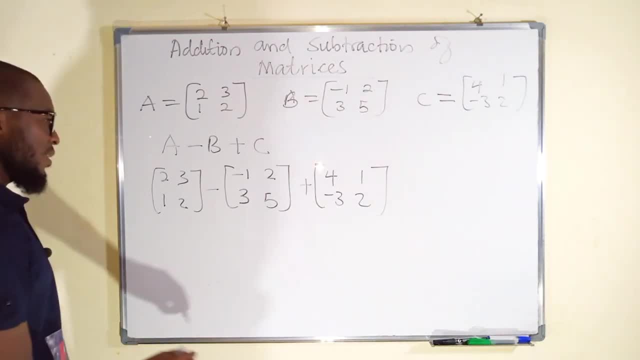 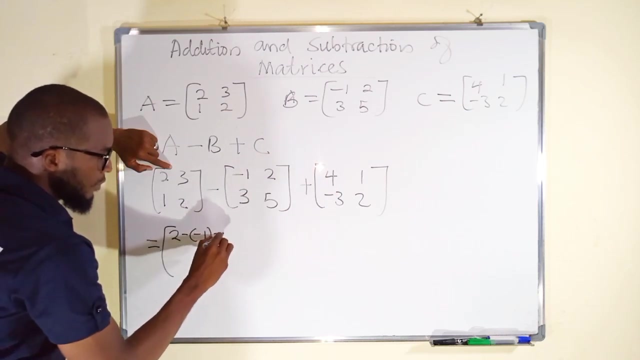 And I think it is the best for me. I can carry them all along. This becomes 2 minus minus 1.. Minus 1. Then plus 4. I can carry them all along. Then you give a space: 3 minus 2 plus 1.. 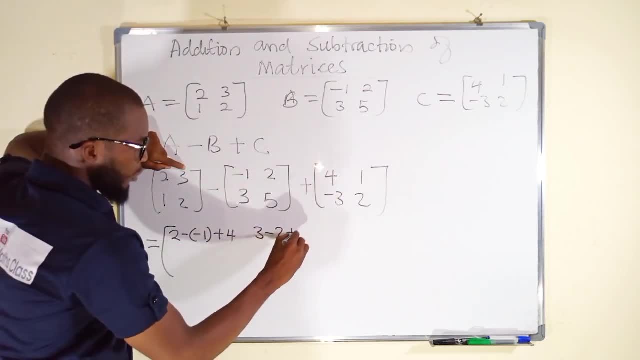 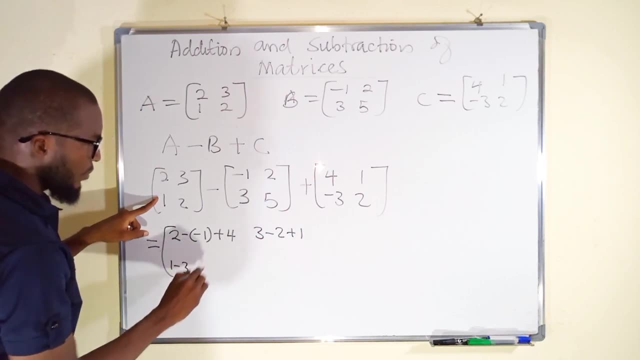 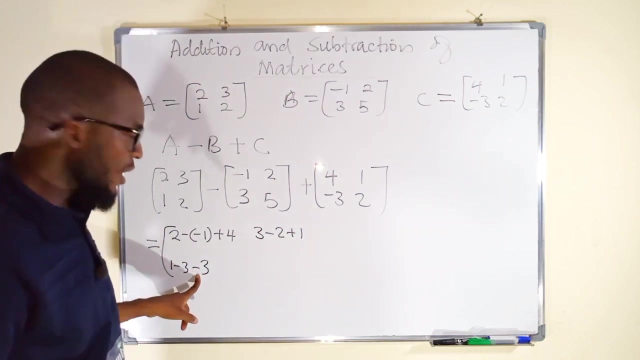 3 minus 2 plus 1.. Then you come here: 1 minus 3.. 1 minus 3.. Then plus minus, So minus is stronger. Therefore we use minus. Then the last element: here We have 2 minus 5.. 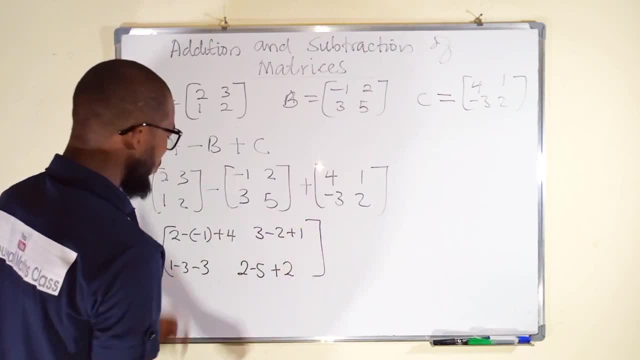 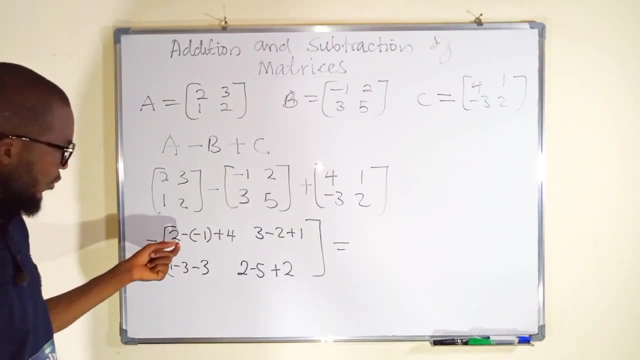 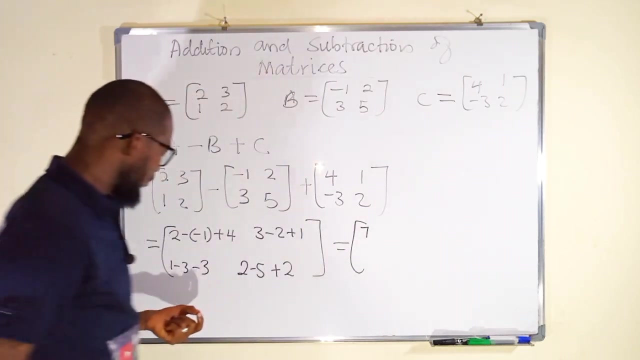 Then plus 2. We close, We simplify To obtain our final result. This is plus because of minus minus. So we have: 2 plus 1 is 3.. Then 3 plus 4 is 7.. We have 7 here. 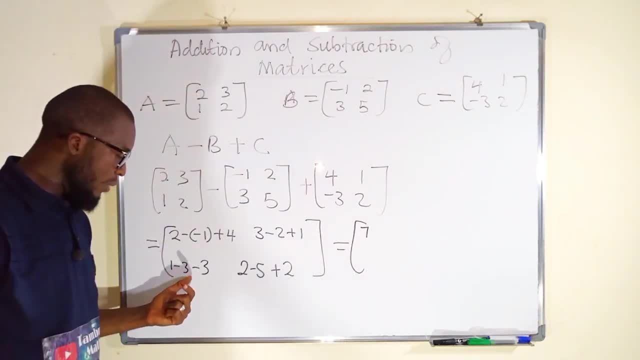 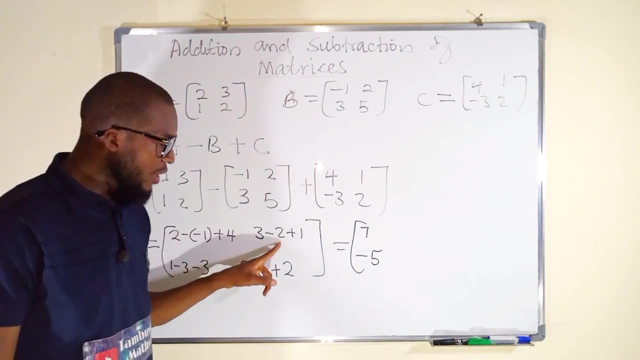 1 minus 3 is minus 2.. Then minus 2 minus 3 is minus 5.. So we have minus 5 here Coming. here We have 3 minus 2 is 1.. Then 1 plus 1 is 2.. 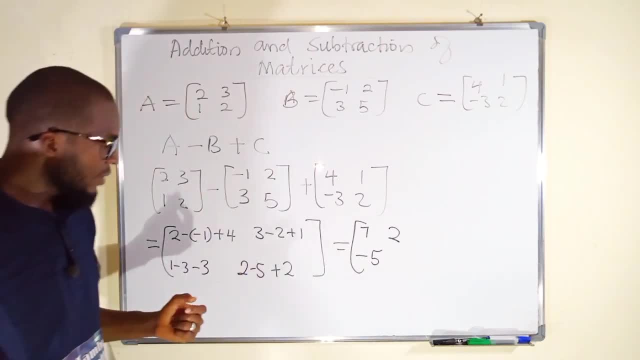 2 minus 5 is minus 3.. Then minus 3 plus 2 is minus 1.. Then minus 3 plus 2 is minus 1.. Then minus 5 is minus 3.. Then minus 3 plus 2 is minus 1.. 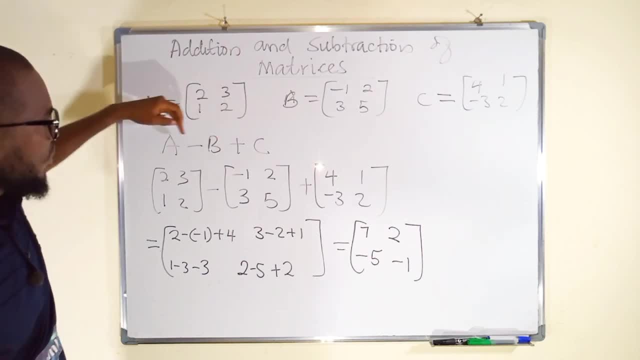 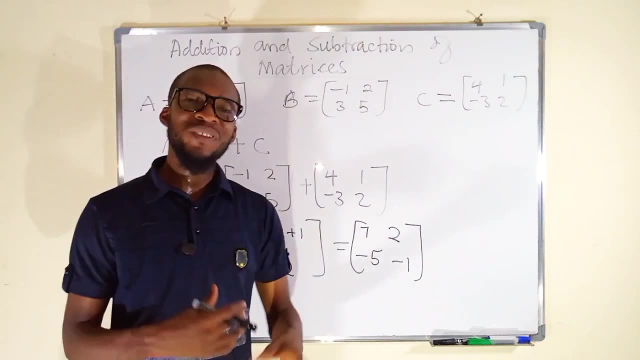 So this is the result After performing this simplification: A minus B plus C. In our next class We are going to look on to scalar multiplication of matrix. We are going to look on to scalar multiplication of matrix. Thank you for watching. Do have a nice day.